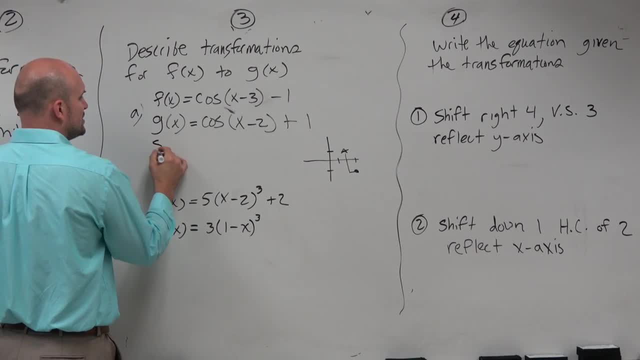 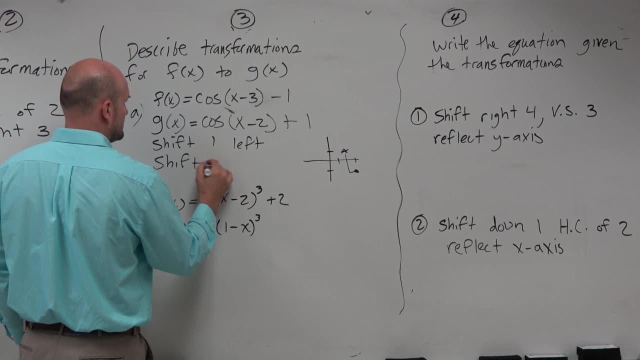 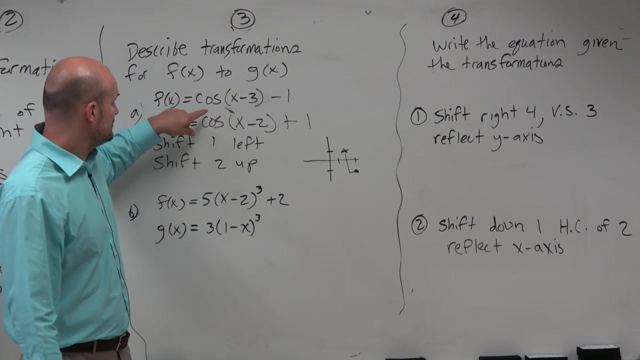 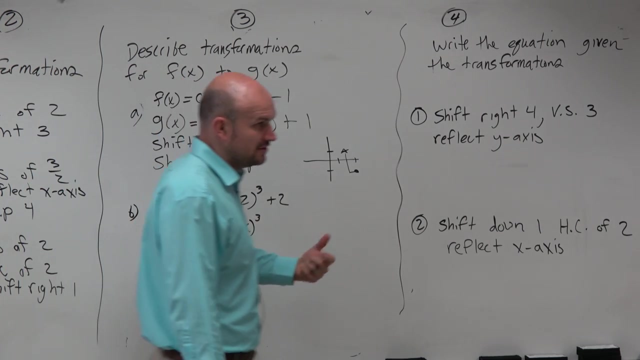 but we understand that the graph. we need to have a shift, one left And shift two up, And if we applied those transformations to this f of x we would get the cosine graph. Now this next one again looks a little bit. 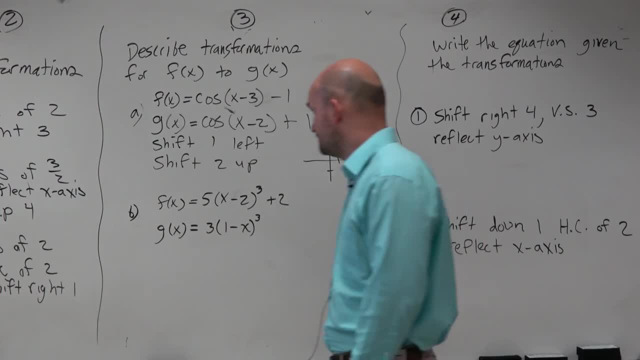 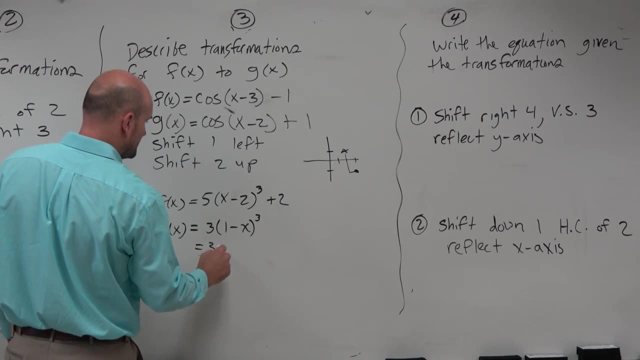 we need to kind of simplify this, because this one's not as straightforward as the other problem. So first thing, I see this and I say, ooh, I got that b right, Just kind of like over here. you've got to simplify it. 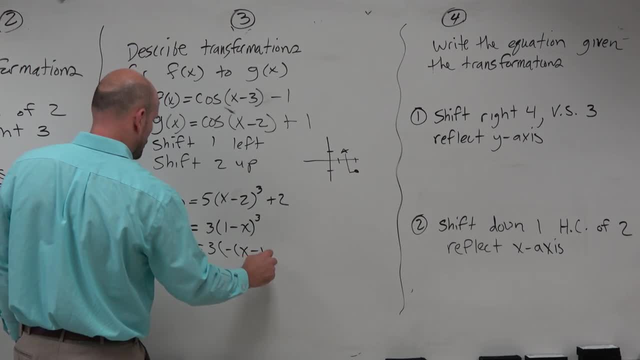 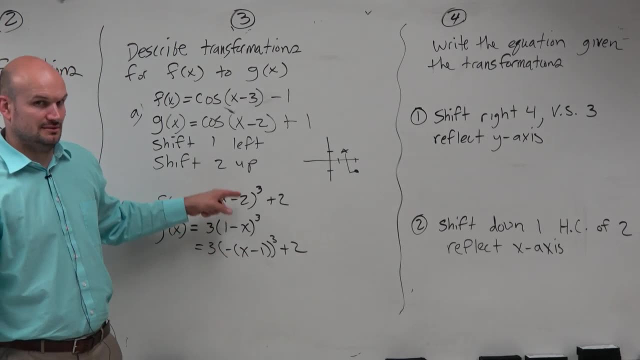 So I'm going to rearrange that and factor out the x. Hopefully you guys are following me here, Not going too fast. Just kind of simplified it and factored it out. I rearranged the terms and then factored it out. 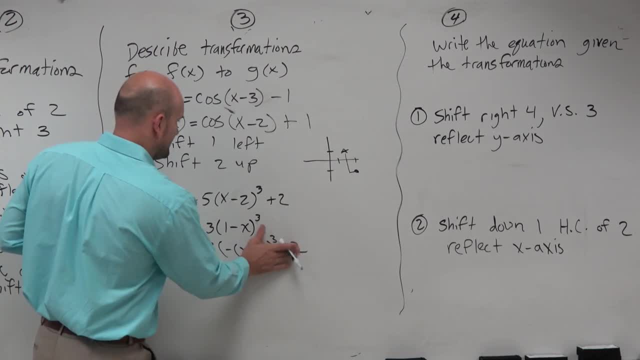 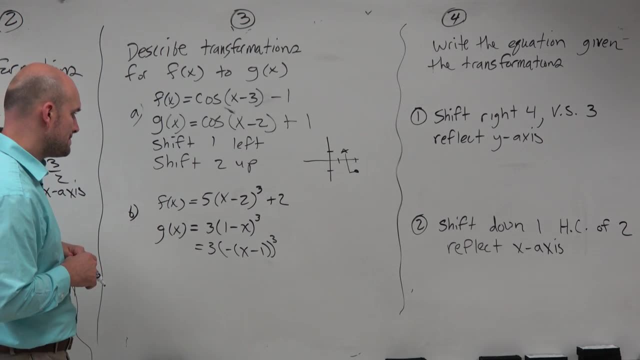 Yes, Where did you get the 2 from? I have no idea. I was grabbing the 2 from there, I guess. All right, So now let's kind of think of this. We have a 5 to a 3.. 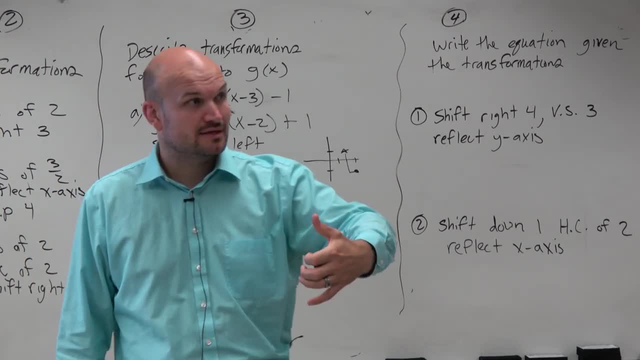 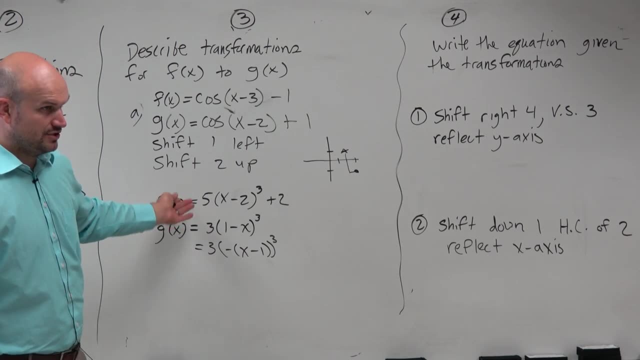 Now again, This is multiplication, right. So you've got to think you were multiplying by 5, and now you're multiplying by 3.. So how do you change this? You don't want to add 2 to it. You've got to think: now multiplication. 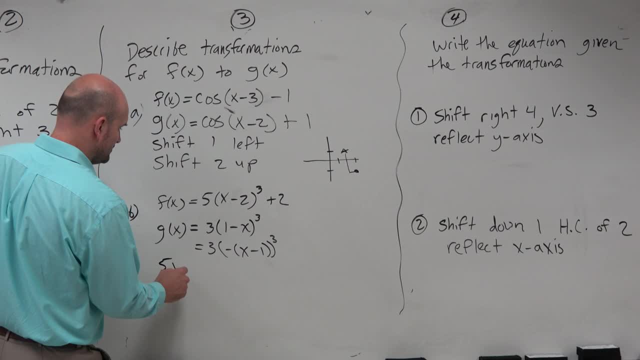 So it's really saying: 5 times what number? Let's use n. 5 times what number equals 3?. Well, if you solve for n, you get n times 3.. That's right, That's right, That's right. 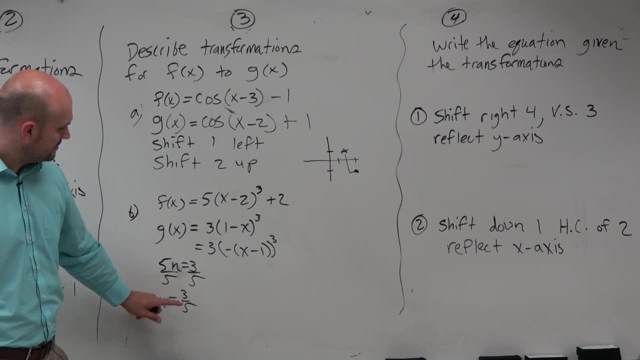 So n equals 3 fifths. Now, is that a compression? If n was equal to again, think about this. Right now, this is a vertical stretch of 5.. Now then it turns to a vertical stretch of 3.. 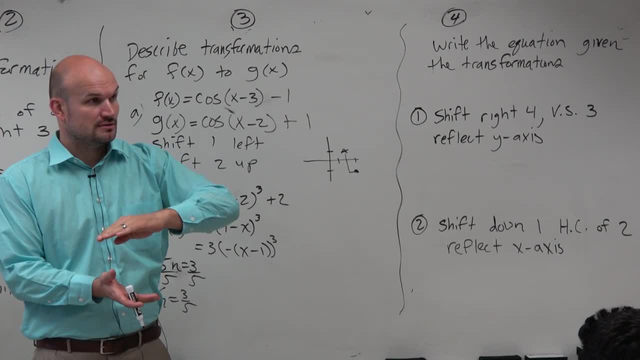 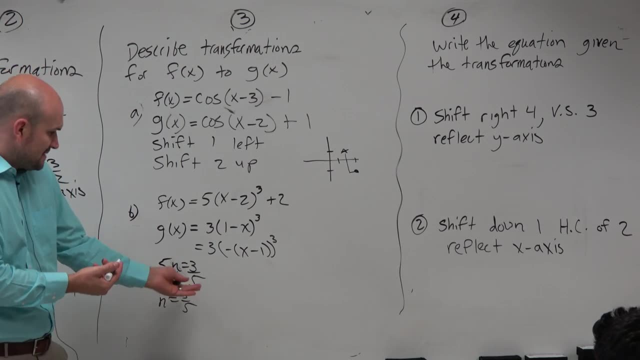 So what happened? Did the stretch get larger or smaller? Smaller? So therefore- and this would make sense- That represents a vertical compression, right, And that makes sense, because that's less than 1.. So we could say that is a vertical compression. 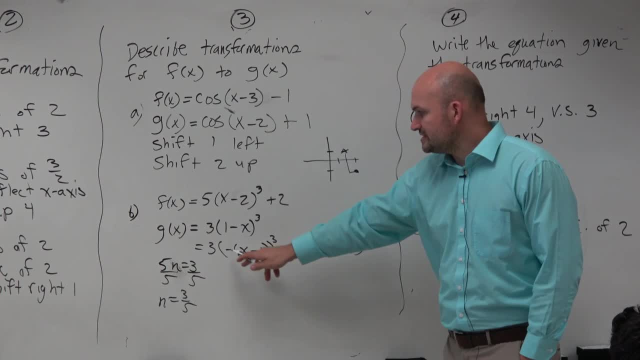 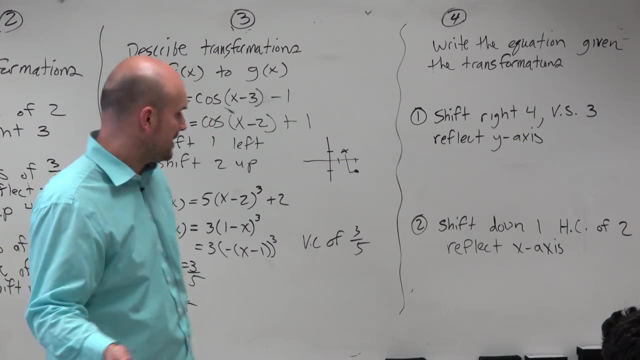 of 3 fifths. You see the negative. There was no negat- there is a negative there and there's a negative there. So the negative didn't change right. So we don't need to add the reflection or change the reflection. 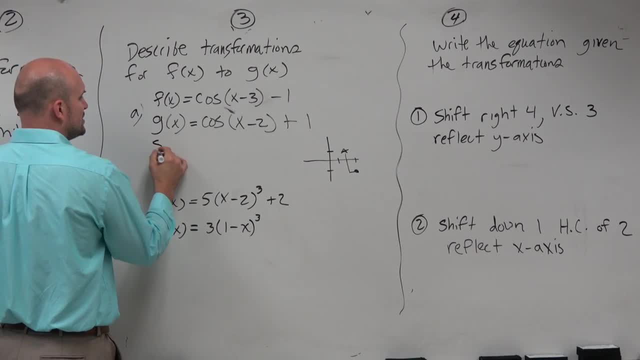 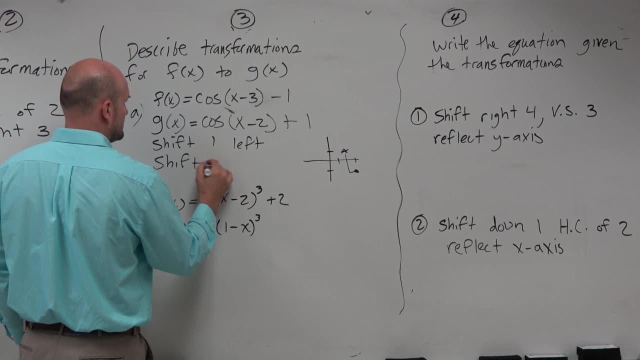 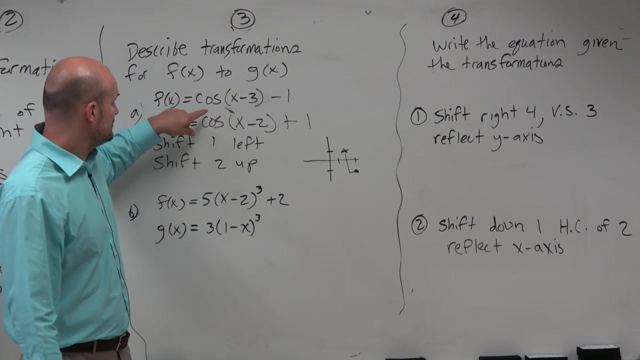 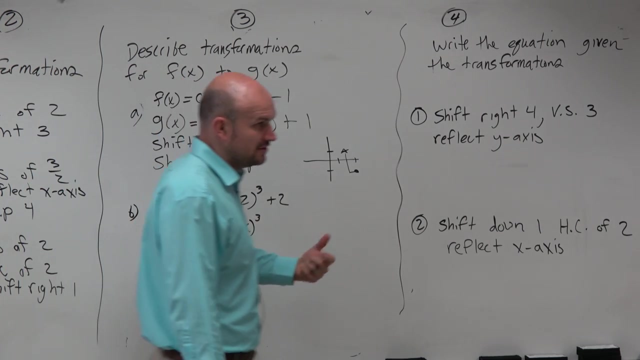 but we understand that the graph. we need to have a shift, one left And shift two up, And if we applied those transformations to this f of x we would get the cosine graph. Now this next one again looks a little bit. 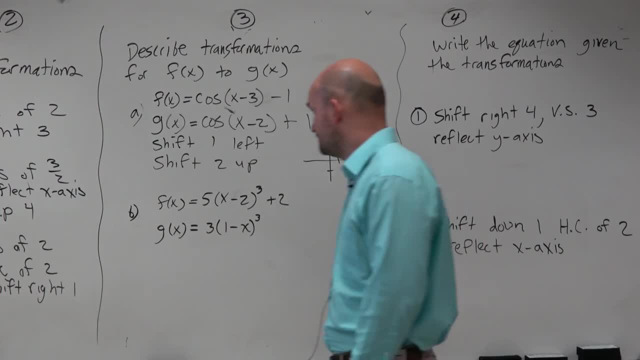 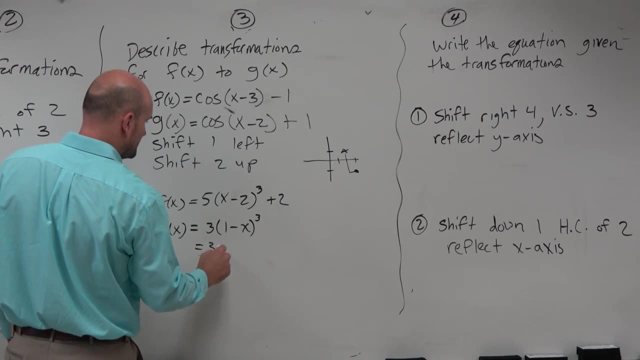 we need to kind of simplify this, because this one's not as straightforward as the other problem. So first thing, I see this and I say, ooh, I got that b right, Just kind of like over here. you've got to simplify it. 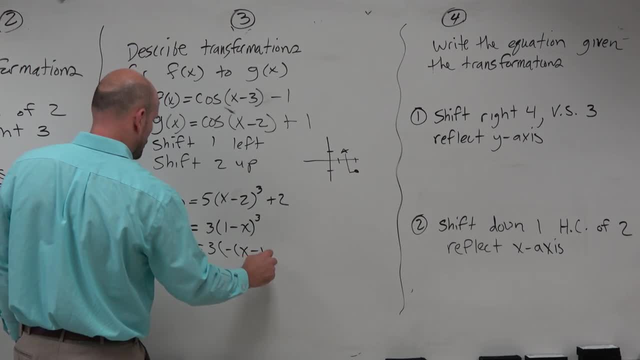 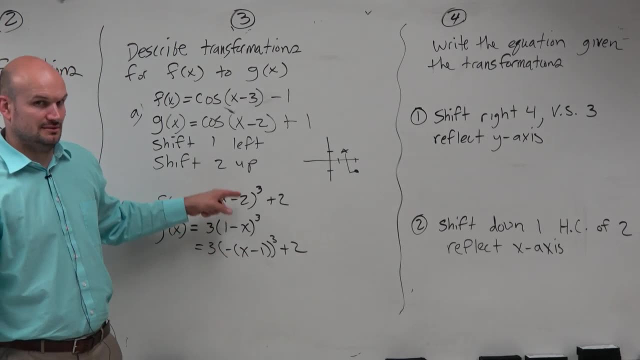 So I'm going to rearrange that and factor out the x. Hopefully you guys are following me here, Not going too fast. Just kind of simplified it and factored it out. I rearranged the terms and then factored it out. 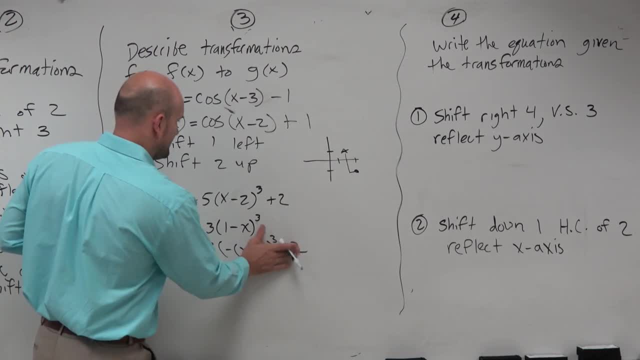 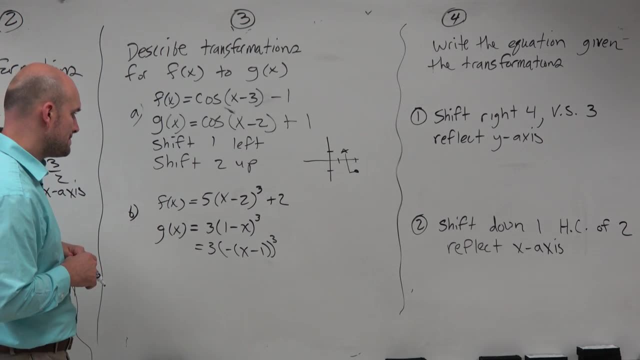 Yes, Where did you get the 2 from? I have no idea. I was grabbing the 2 from there, I guess. All right, So now let's kind of think of this. We have a 5 to a 3.. 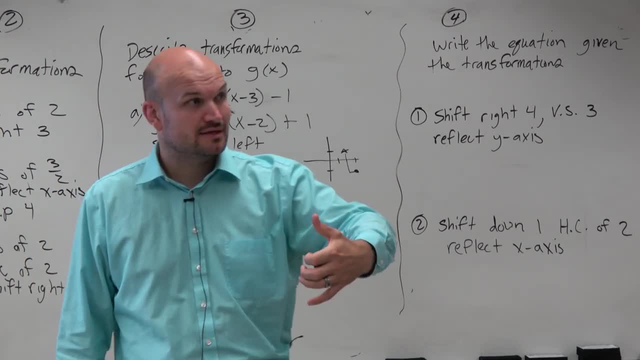 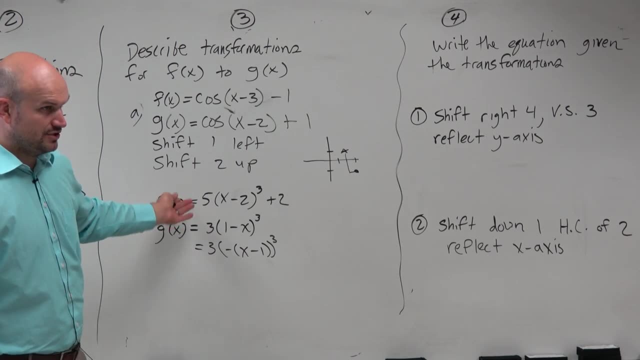 Now again, This is multiplication, right. So you've got to think you were multiplying by 5, and now you're multiplying by 3.. So how do you change this? You don't want to add 2 to it. You've got to think: now multiplication. 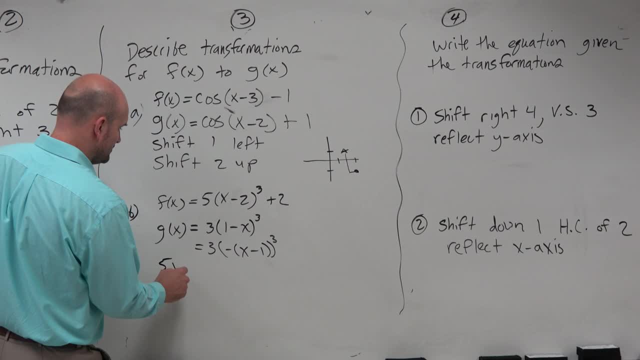 So it's really saying: 5 times what number? Let's use n. 5 times what number equals 3?. Well, if you solve for n, you get n times 3.. That's right, That's right, That's right. 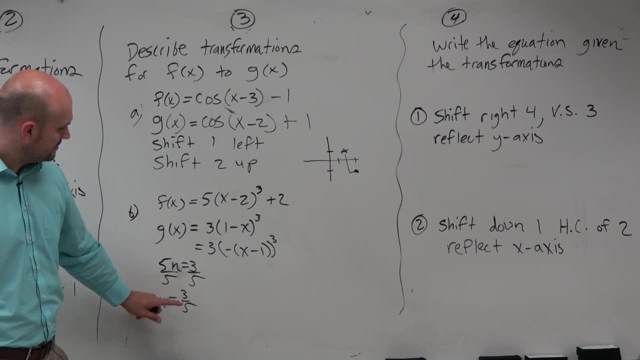 So n equals 3 fifths. Now, is that a compression? If n was equal to again, think about this. Right now, this is a vertical stretch of 5.. Now then it turns to a vertical stretch of 3.. 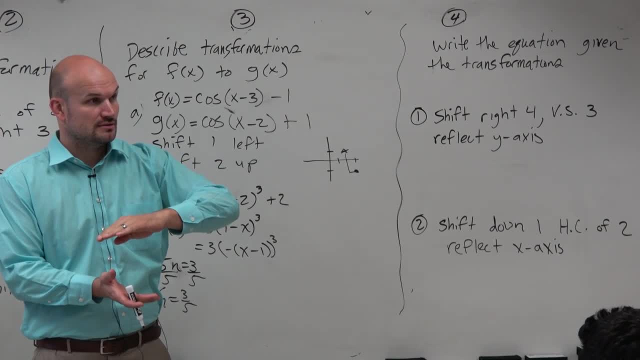 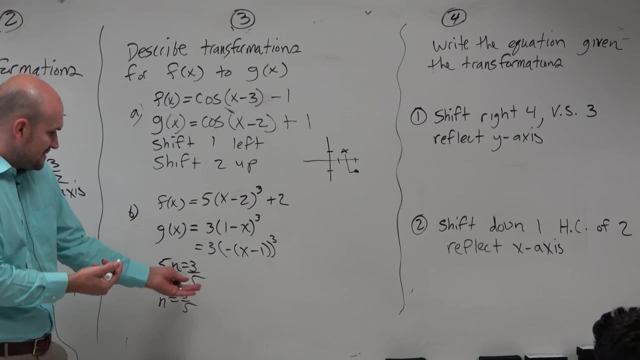 So what happened? Did the stretch get larger or smaller? Smaller? So therefore- and this would make sense- That represents a vertical compression, right, And that makes sense, because that's less than 1.. So we could say that is a vertical compression. 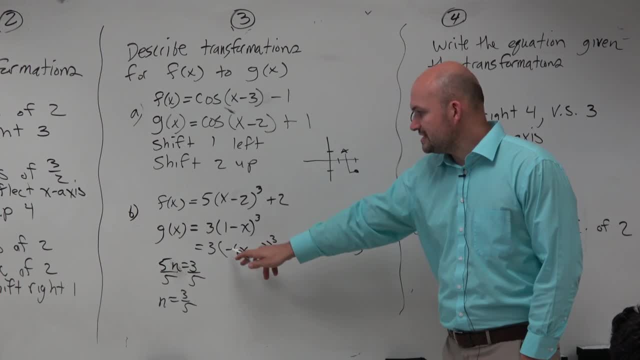 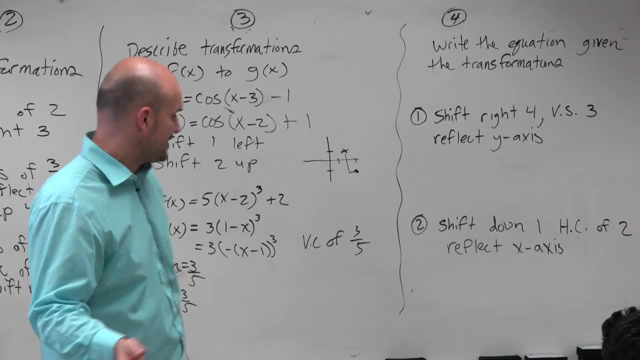 of 3 fifths. You see the negative. There is a negative there and there's a negative there. So the negative didn't change right. So we don't need to add the reflection or change the reflection. I'm sorry.